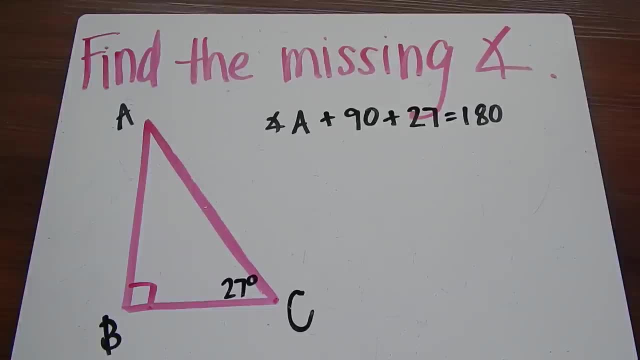 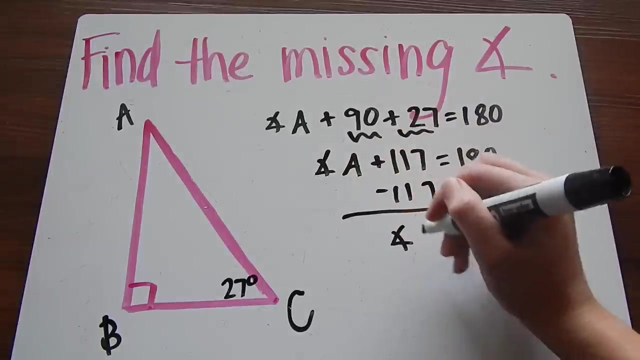 That is right. That is right. That is the theorem that we just talked about And now we need to solve. So angle A- I'm going to combine like terms here- 90 plus 27 is 117, equals 180.. Subtract 117 from both sides And we have angle A is equal to 60. 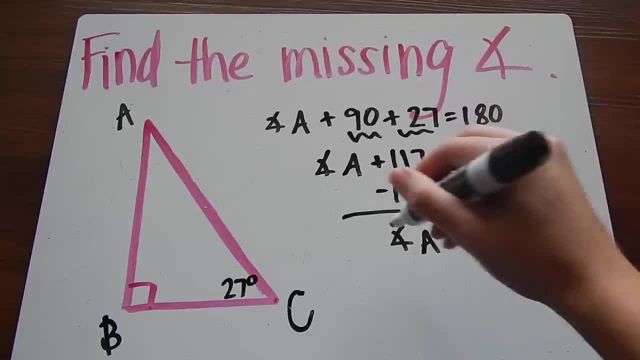 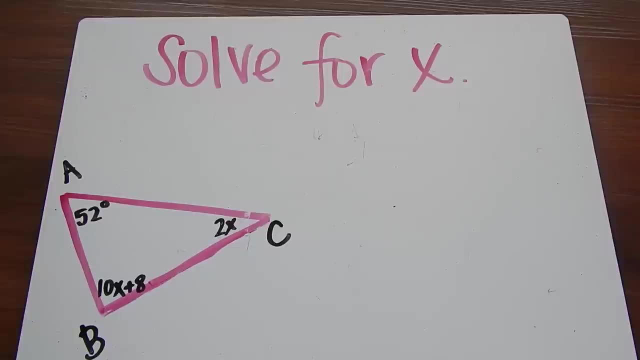 And that is our answer. Okay, next problem. This one says solve for X. So again, I'm going to add all the angles together, set it equal to 180.. So it's going to be 52 plus 10X plus 8 plus 2X equals 180. 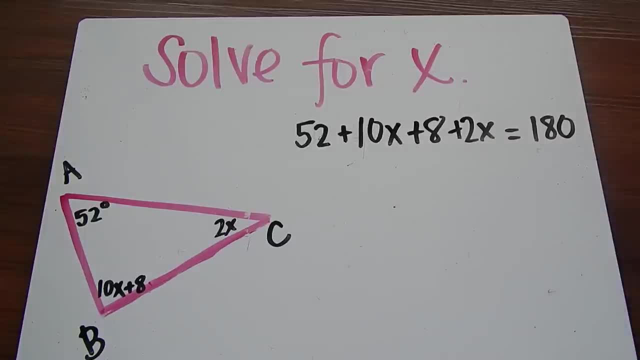 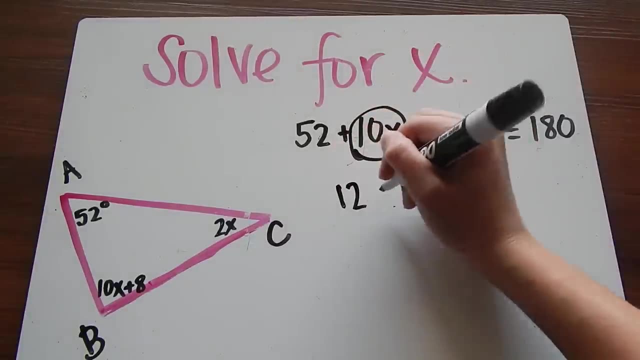 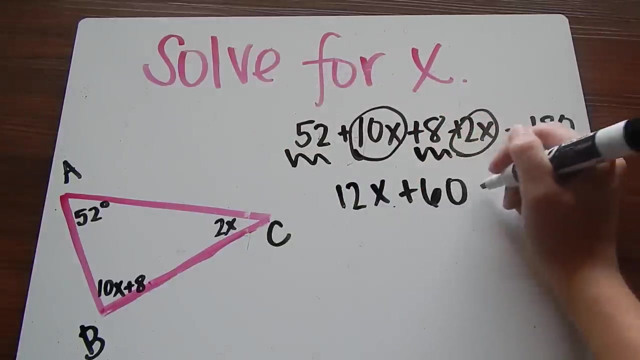 Here's A plus B plus C. Now we want to combine like terms, So I'm going to add all the X's together: 10X plus 2X is 12X. Add the numbers together: 52 plus 8 is 60. And we'll just solve for X. I'm going to subtract 60 from both sides. 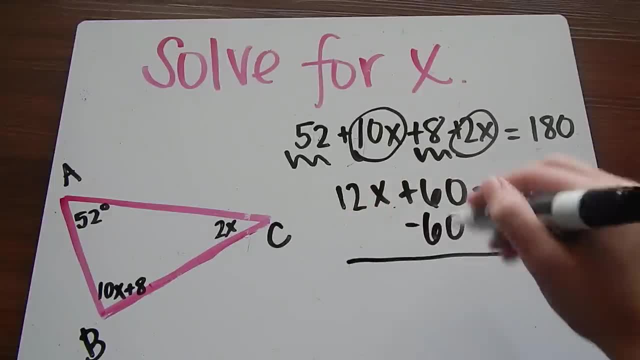 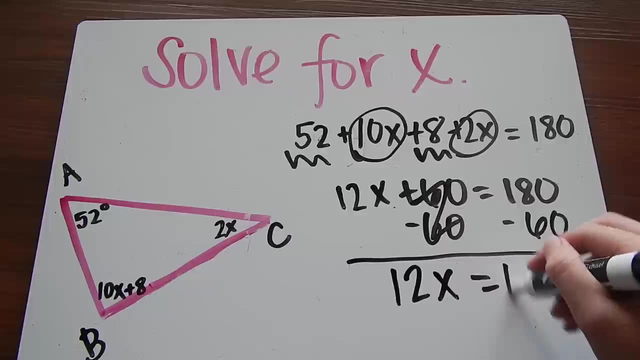 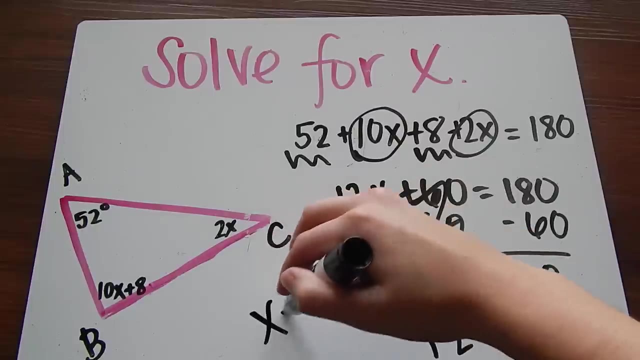 And we'll just solve for X. I'm going to subtract 60 from both sides, And we'll just solve for X. I'm going to subtract 60 from both sides. I get 12X equals 180 minus 60 is 120.. Divide both sides by 12. And I get my answer: X equals 10.. 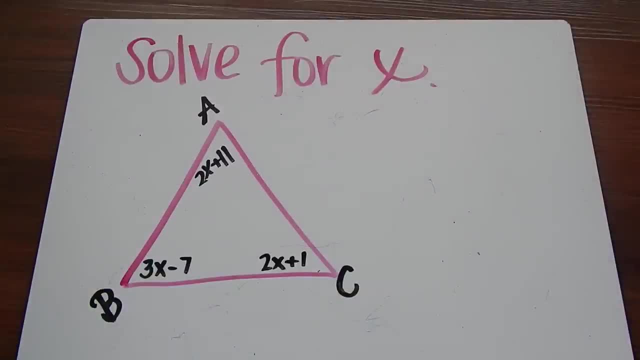 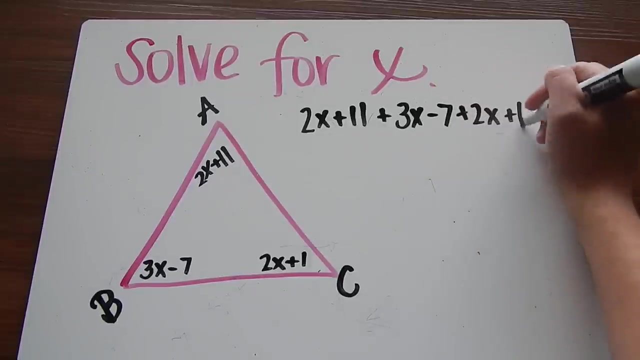 And our last example: here Again we're going to solve for X. So again we're going to take each angle measure and add them together. Set it equal to 180.. So we'll have A, which is 2X plus 11,, plus B, which is 3X minus 7,, plus C, which is 2X plus 1, equals 180.. 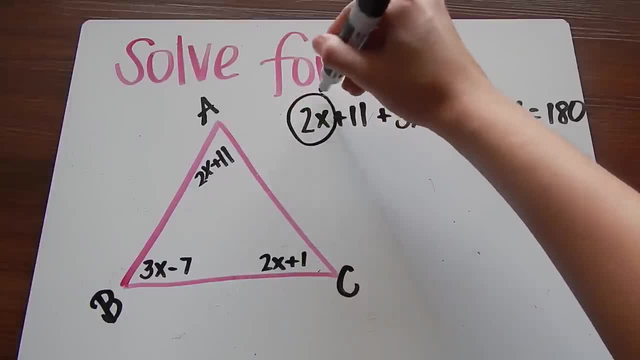 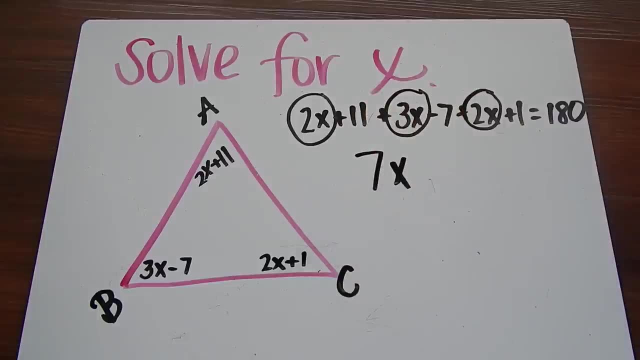 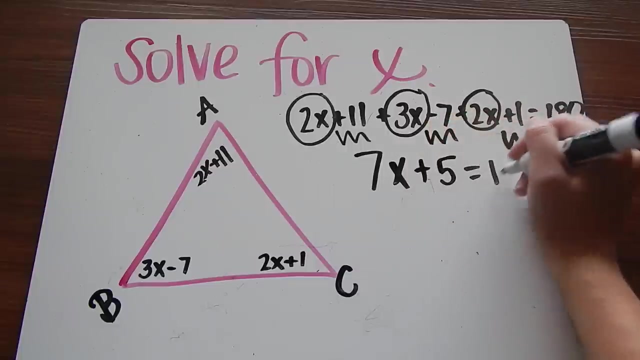 Combine like terms. So I'm going to add up all my X's: 2 plus 3 is 5, plus 2 more is 7.. So 7. 7X. And then add all my numbers: 11 minus 7 is 4, plus 1 is 5.. It's a positive 5, so it's going to be plus 5..